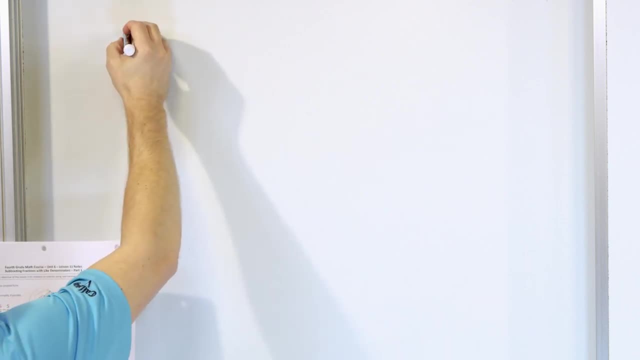 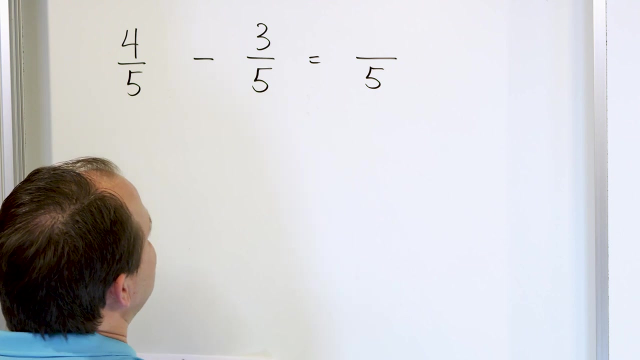 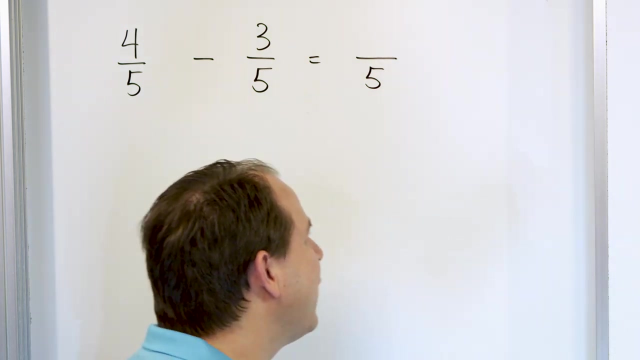 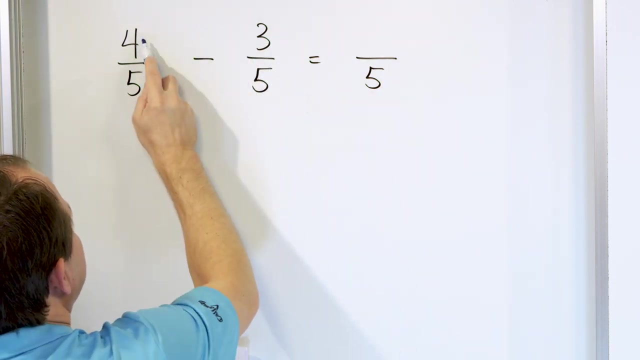 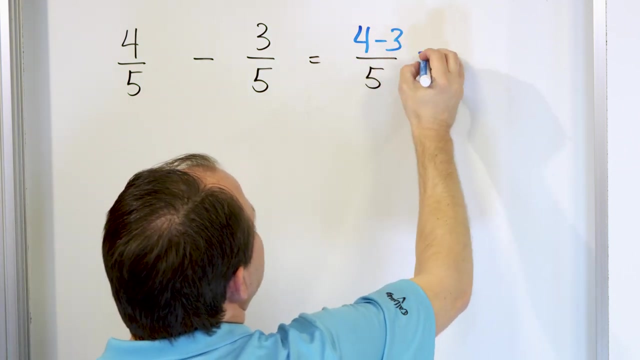 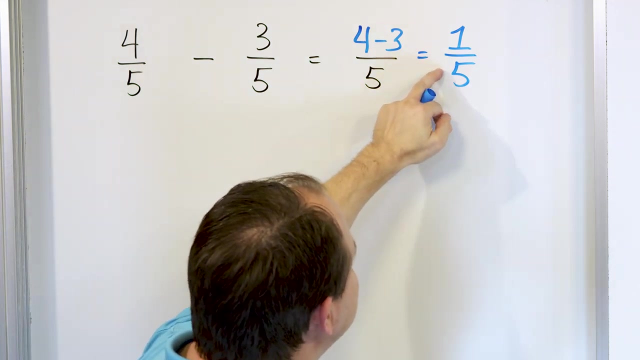 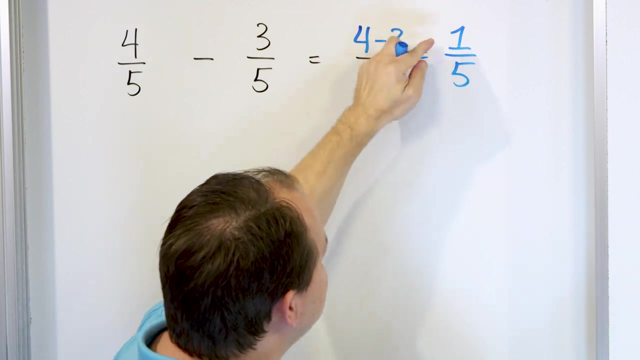 We can understand what's going on. Let's take a look at the fraction four-fifths, and we want to subtract from that the fraction three-fifths. So the first thing we do is we check, are the denominators the same? In order to add or subtract fractions, the denominators must be the same. We'll talk a little bit more about why in just a minute, but for now, keep the denominator the same in your answer. The denominator has to be a five. You do not subtract the denominators. You keep the same denominators. You keep the same denominators, the denominator in your answer, just like for adding. We keep it here. Now, in the numerator, which is the top, we have a four and a three, but we have a minus sign, so it's four minus three. So instead of adding them, we basically subtract them. It's very, very simple. Four minus three, as you know, is one, and then, of course, five stays along for the ride, one-fifth. And then we ask ourselves, can we simplify this fraction by dividing the top and the bottom of the fraction by the same number? We really can't do anything. 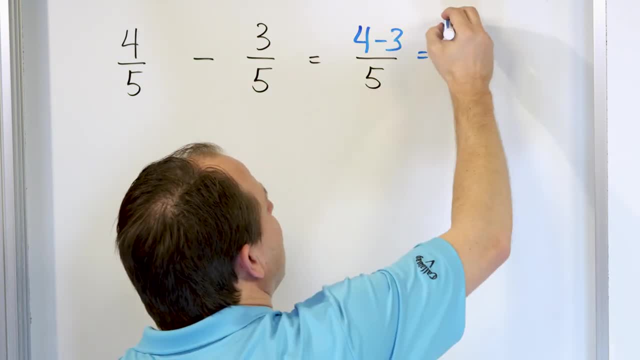 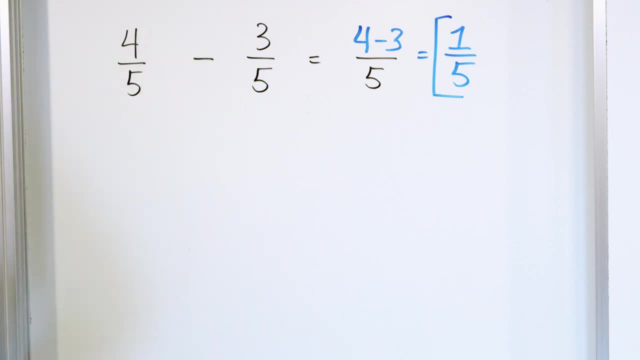 Divide top and bottom by anything that's going to make these numbers any smaller. So one-fifth is the final answer. So let's talk about why this makes sense, right? So here we have four out of five pieces of a pizza. So we have a pizza cut into, let's go ahead and call it five pieces. So one-fifth, two-fifths, three-fifths, four-fifths. Here is five-fifths. That's what we have, a pizza cut into five pieces. But here we have four of those five pieces, one, two, three, four. That's what we have here. This is how much pizza we have. 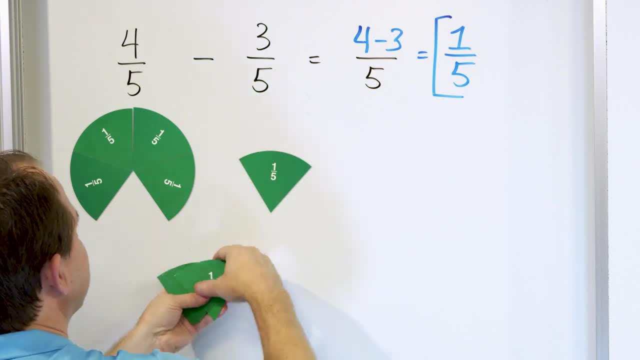 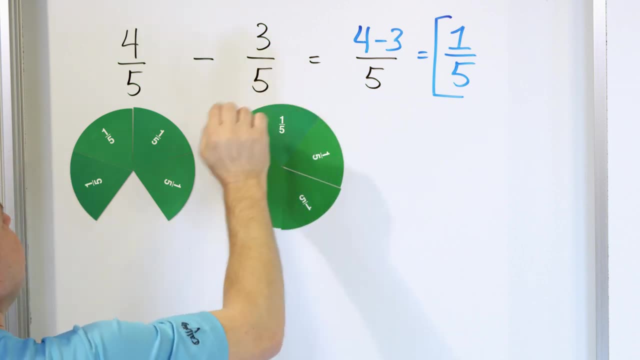 Now here we have three out of five pieces of a pizza. So let's build another pizza. There's one, there's two, there's three, there's four, and there's five. So here's another pizza, again, cut into five pieces, but here I only have three of them, one, two, three. So what we're saying is we have four out of five pieces of a pizza, and here we have three out of five pieces of a pizza, but instead of adding them together, making it larger, what we're going to do is subtract them. 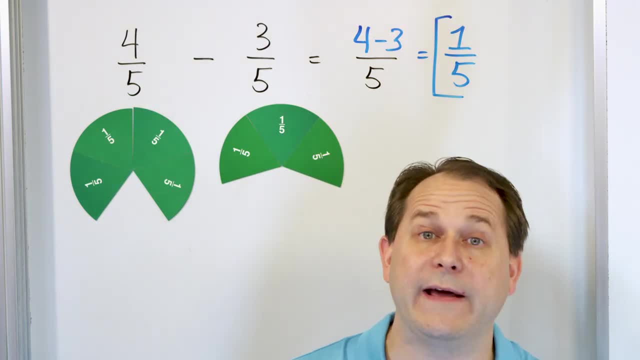 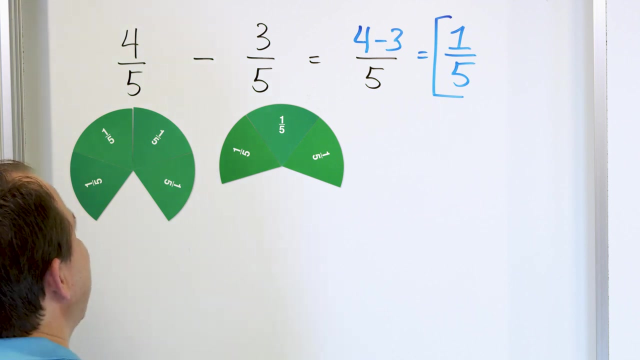 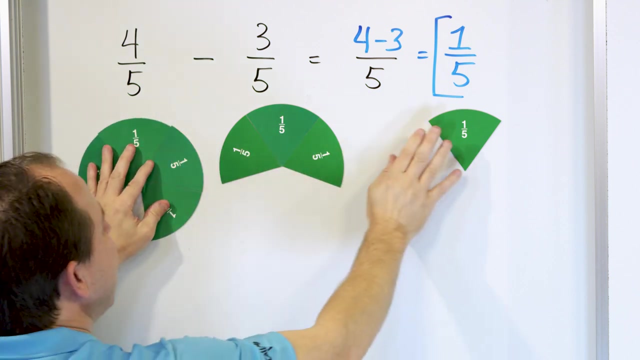 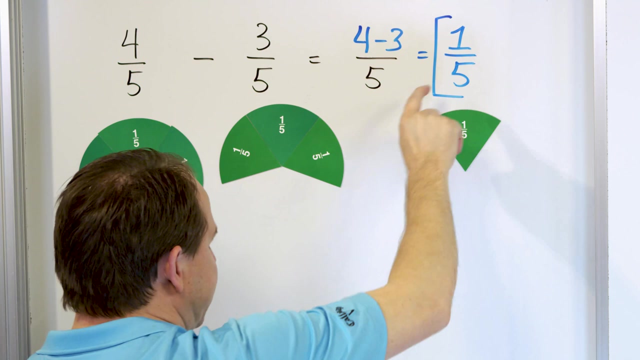 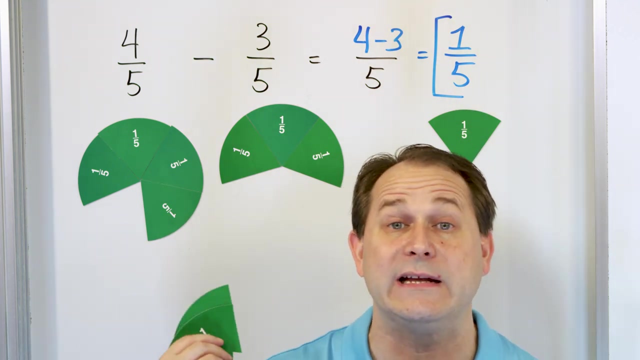 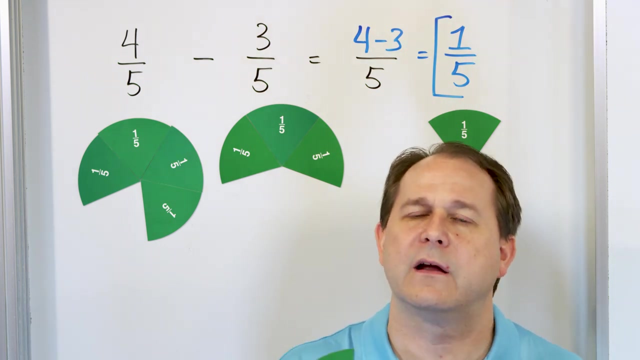 Think about it. If you have four pieces of something, and you take away three pieces of something, then you only have one piece left. And here we're saying we have four pieces of pizza. The five tells us how big the slices are, basically. We have four of them here, and we have three of them here. We subtract them, and so what we actually get when we subtract them, four minus three is one, which is the answer, one-fifth here. Because if we start with this, and we take away three of those pieces like this, what are we left with? Only one piece left. Addition would be if we add these together, subtraction is we take this amount, and we take it away. We only have that one piece left. So we have one-fifth there. So that's why when we check to make sure the denominators are the same, we keep the same denominator in our answer. Because I've been telling you before that I want you to start viewing these fraction wedges as things that you can count. You don't really want to add or subtract wedges of different sizes. I mean, you could, but they're different. They won't make a lot of sense to add one-third or subtract one-third. So you want to start with one-third and one-fourth, because the size of the slices there would be different. Here, all the slices are the same thing, so it's a simple matter of just subtracting them or adding 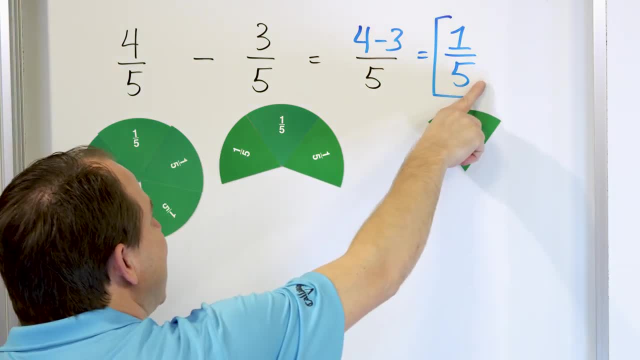 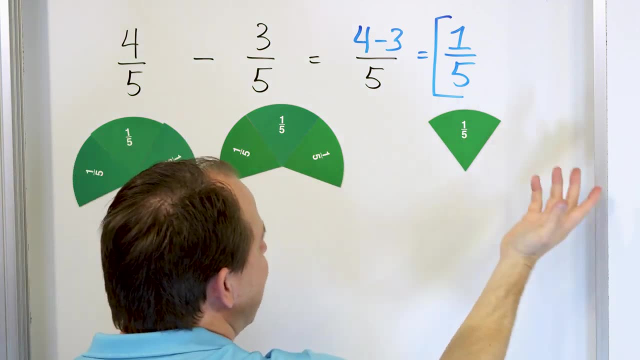 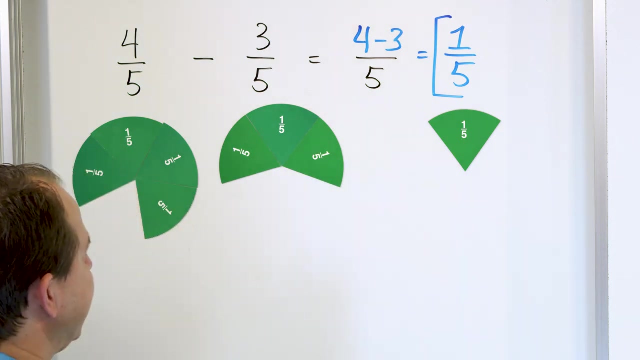 them together. That's why we keep the same denominator in the same, because here we have four out of five pieces. We take away three out of those five pieces. How many do we have left? One out of five pieces of the pizza there. And of course, we try to simplify that, and we really can't simplify any further, so we're done, right? All right, let's go on. I'm 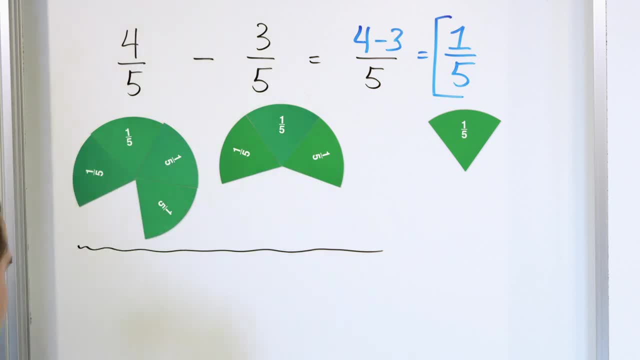 going to leave this up here. We'll kind of refer back to it later. Let's take a look at the next problem. Let's say we have three-fourths, and we want to subtract from it one-fourth. 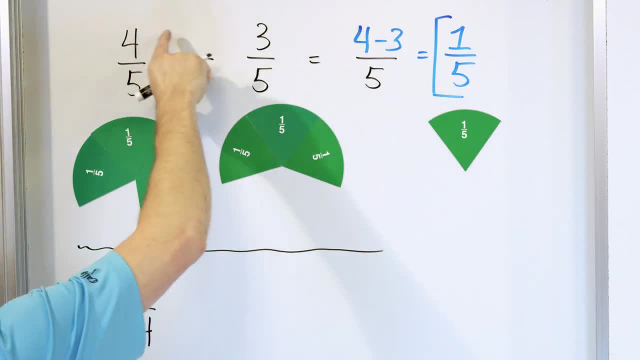 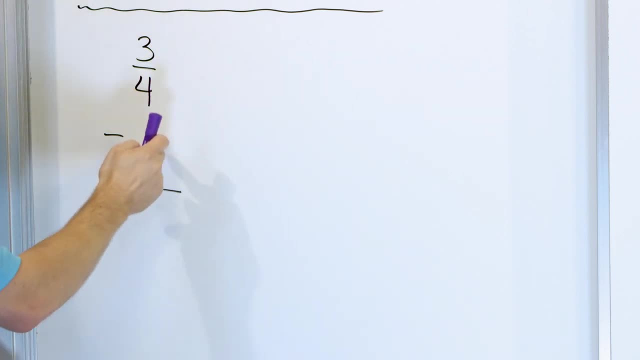 Now again, the first problem had the problem written on its side horizontal like this. You can also see the problems stacked on top of each other. It's fine either way. Now we check. Four and four, those are the denominators. So we keep the same denominator. 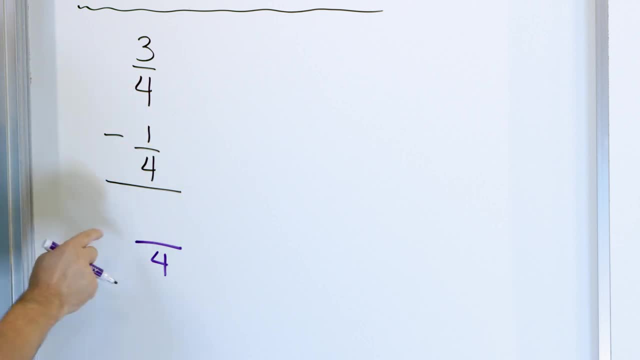 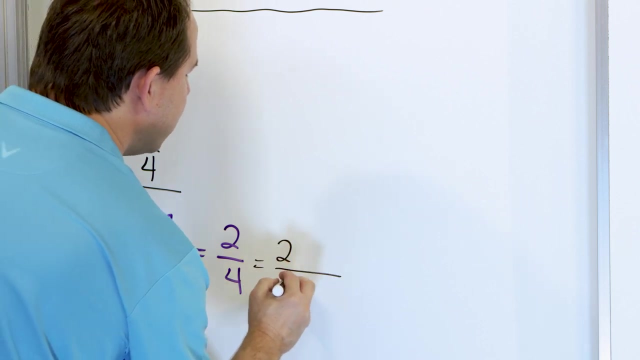 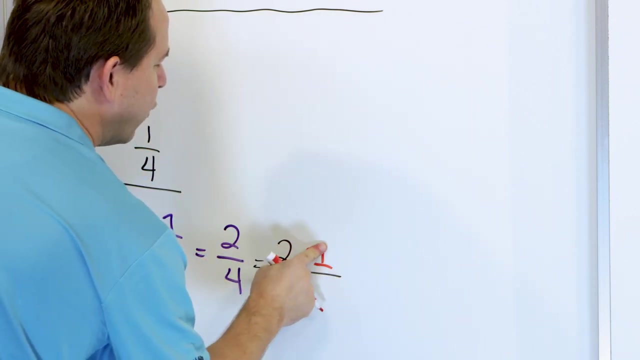 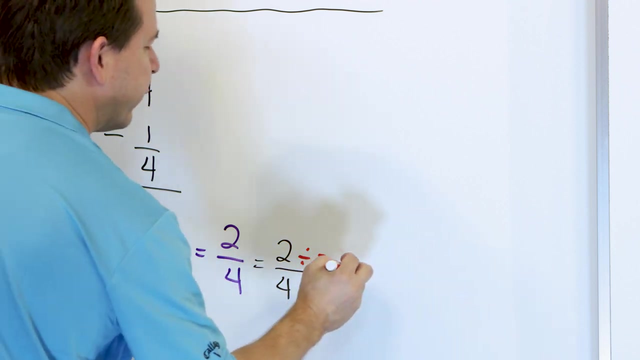 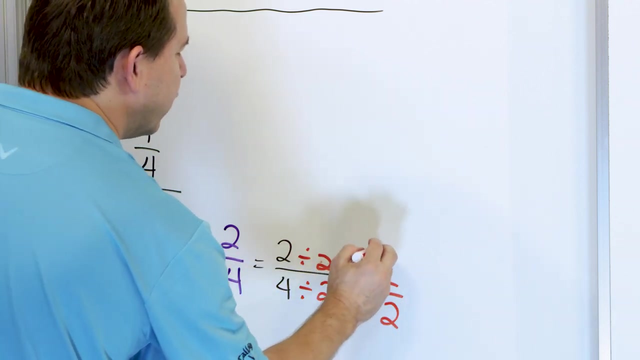 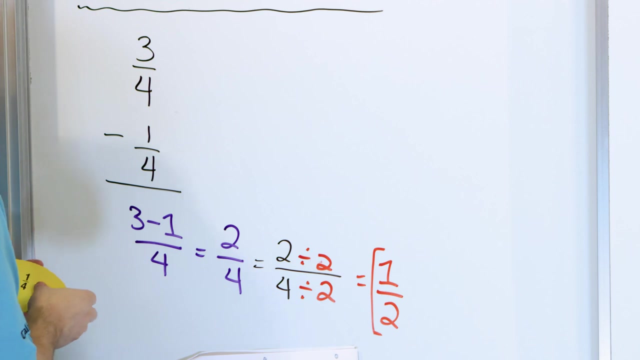 We don't subtract them. We don't add them. We keep the same denominator. There's a four down here. What do we have on top? Three minus, because there's a minus one. Three minus one. That goes in the numerator. Instead of adding them, we subtract them. Three minus one is two, two out of four pieces. Now, what this is telling us is if we have three out of four pieces of a pizza, and we take away from that one out of four pieces, then we should have two pieces left over. Three pieces minus one piece should give us two pieces out of four, which tells us how big the slices are there. But we check. Is this fully simplified? No, it's not, because we can divide the top and the bottom by 2, because those are both even numbers. So let's take and divide the top by 1. I'm sorry, not by 1. We're going to divide the top by 2, and we'll also divide the bottom by 2. We divide top and bottom by whatever we want. 2 divided by 2 is 1, and 4 divided by 2 is 2. 2 times 2 is 4. 1 times 2 is 2. So we think the answer is 1 half. Does this make any sense? Let's check it out. Let's build this here. What we're saying is that this is 1 fourth of a pizza, 2 fourths of a pizza, 3 fourths of a pizza, and 4 fourths of a pizza. We've cut a pizza into 4 equal slices, but we only have 3 of those slices, so this is actually how much 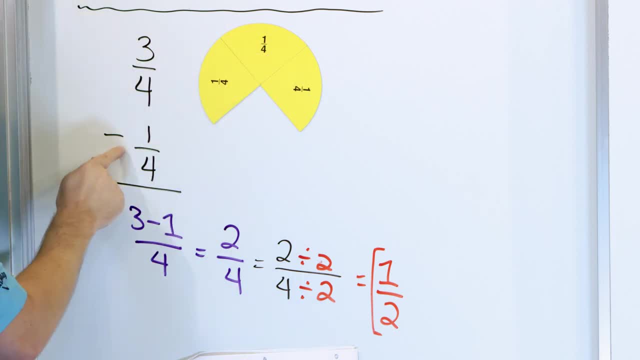 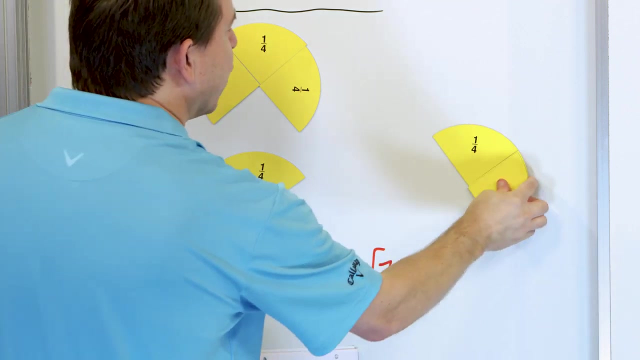 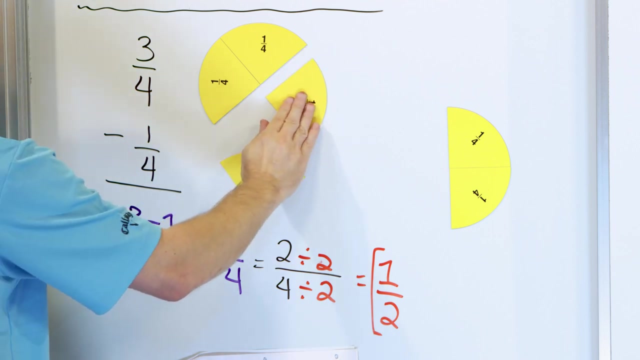 pizza we have in the top fraction. The bottom fraction is 1 fourth. That is this amount of the pizza, 1 out of 4 slices. Instead of adding them together, if we add them together, we would just put it over here. It would actually make a whole pizza if we add them together. But we're not. We're taking away one slice from here. So it's like you take away one slice. What do you have left? You have this. You have 1 fourth, 2 fourths. So we have 1 fourth, 2 fourths. This is what you get whenever you subtract it, because if you start with 3 out of 4 pieces and you take one of these away, you have this much left, which is 2 out of 4 pieces. But you can see right away that 2 out of 4 pieces of anything is exactly the same as 1 half. You can actually see it represents the same amount. 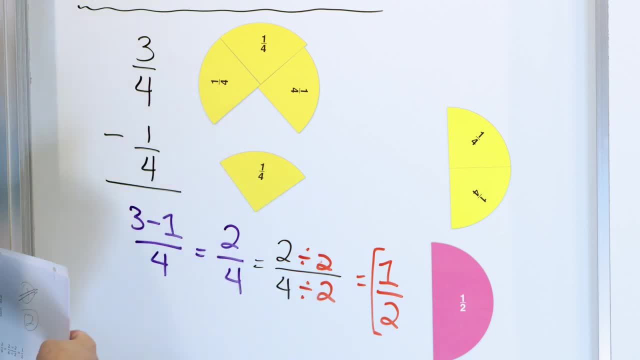 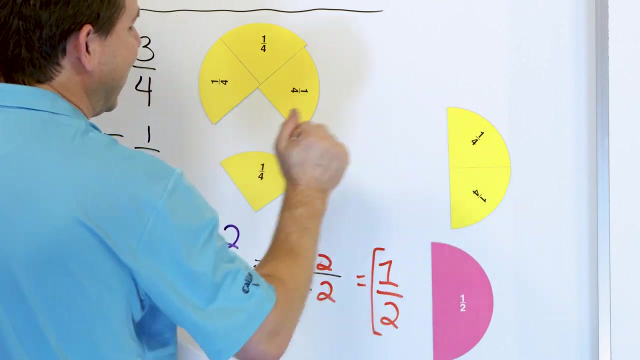 So the answer is 2 fourths. That's correct. That's a perfectly fine way of saying it. If you start with 3 pieces and you take away 1 piece, you should only have 2 pieces left out of 4 pieces of the pizza, sliced into 4 slices. But a simpler way to write it is as 1 half. This represents the exact same amount of pizza as that. 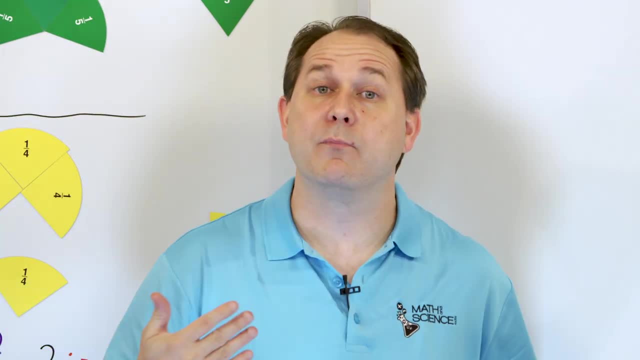 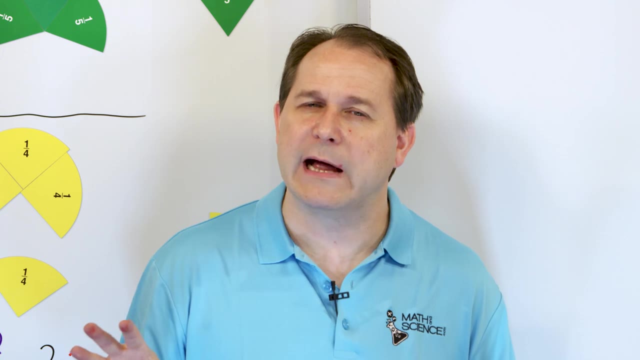 So I think I'll do 1 or maybe 2 more where we use our magnets, but more or less now I want to take the training wheels off and just solve the problems without using the magnets. They're really good to visualize, but we do have to get good at doing this without putting magnets in place and counting anything. 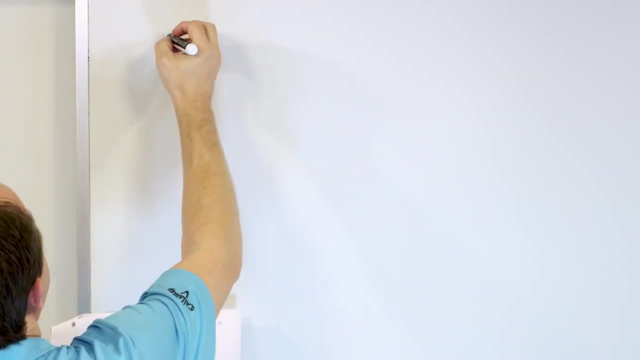 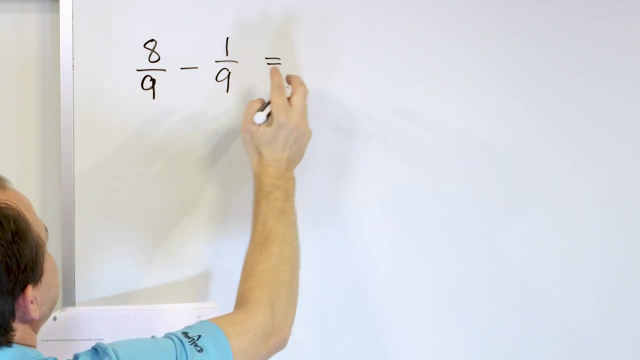 So what do we have? Next problem is going to be 8 ninths, and we're going to subtract 1 ninth. We're subtracting fractions. The denominators must be the same, and they are. 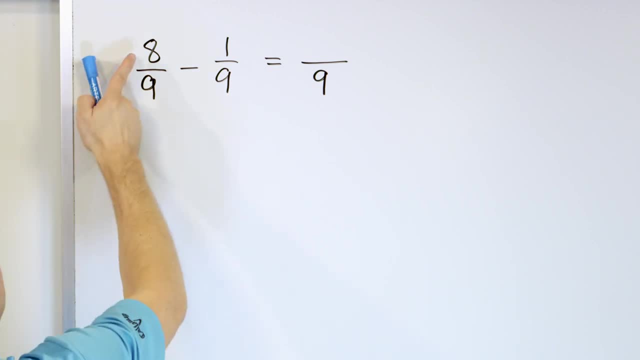 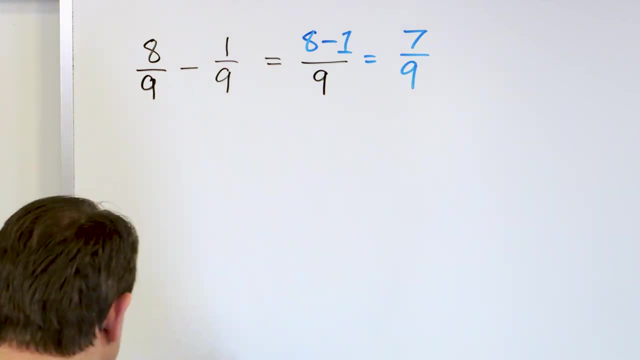 But again, 8 minus 1 is 7, and it's out of 9 pieces. So if you start with 8 out of 9 pieces, and you take away 1 out of 9 pieces, then you're only going to have 7 pieces left, of course, out of 9, 7 ninths. And you cannot simplify this any further, because you can't divide top and bottom by anything to make that simpler. So we just say that's the final answer. 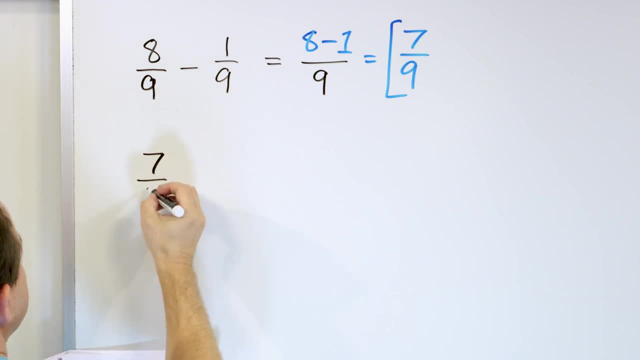 All right, problem number 4. Let's say we have 7 tenths, and we're subtracting from that 4 tenths. 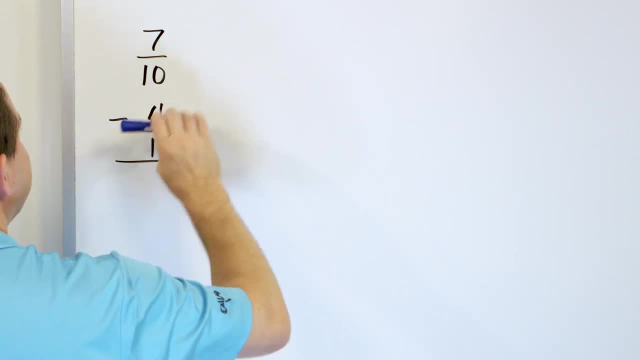 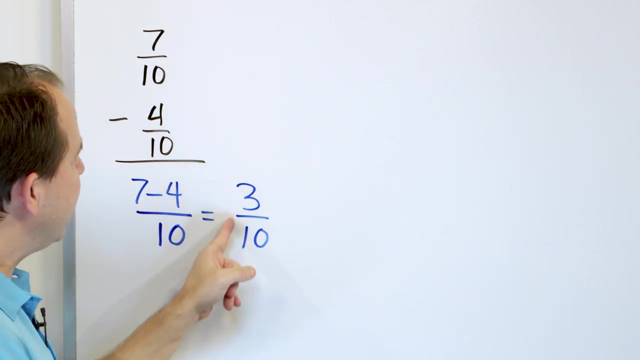 All right, what do we have? The denominators here, 10 and 10. They're the same denominator, so we keep the same denominator in the answer. And we have a 7 and a 4, and of course, they're subtracted. So the numerator is 7 minus 4. What do we get? 7 minus 4 is 3, and so it's 3 out of 10 pieces. 3 out of 10 pieces. So it makes sense. If you start with 7 out of 10 pieces of a pizza, and you take away 4 slices, you start with 7 slices and you take away 4 slices, you should get, have 3 slices left, of course, out of 10. And so, is this fully simplified? Can we divide top and bottom by something to make it simpler? And we can't, because this is an odd number and this is an even number, and we can't divide top and bottom by 2 or by 3 or anything else, so it's just 3 out of 10. 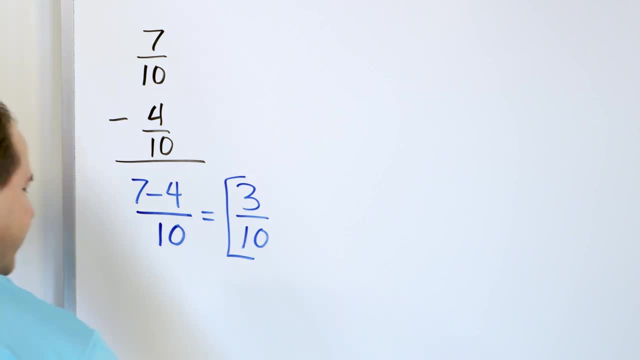 Now, this will be the last problem where I kind of use the magnets to help us kind of visualize. I do think it's worth doing, but after this one, we're not going to basically do this anymore. 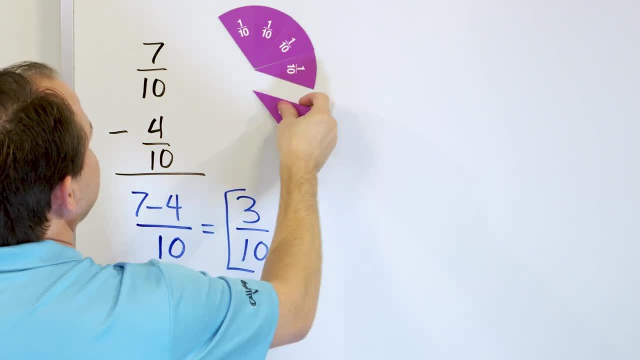 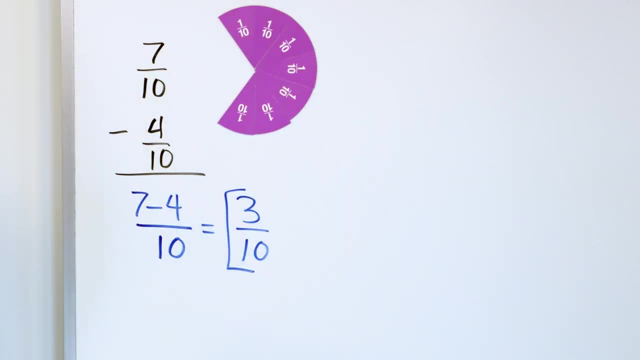 So there's 1 tenth, 2 tenths, 3 tenths, 4 tenths. Here's 5 tenths. Here's 7 tenths. 6 tenths. There is 7 tenths. So this is the amount of pizza represented by this fraction. 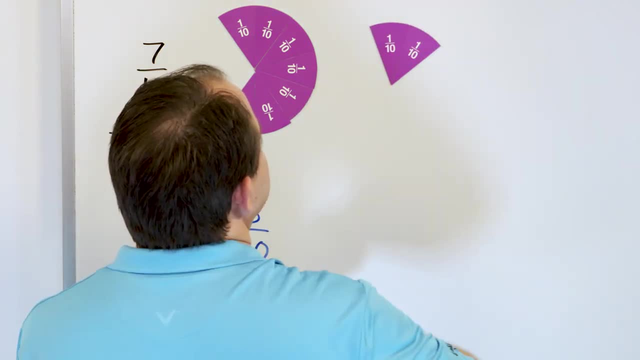 This is 4 tenths. 1 tenth, 2 tenths, 3 tenths, 4 tenths. 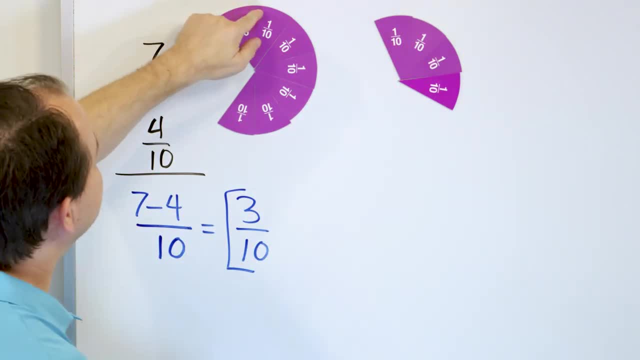 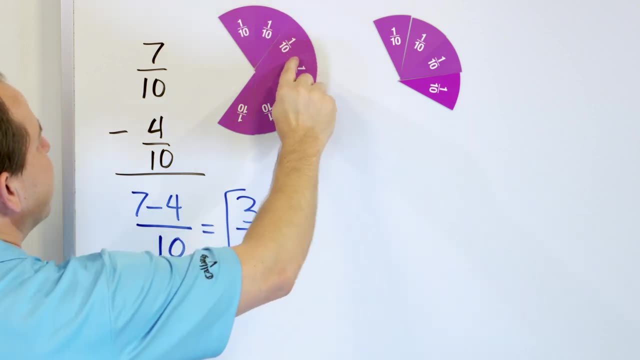 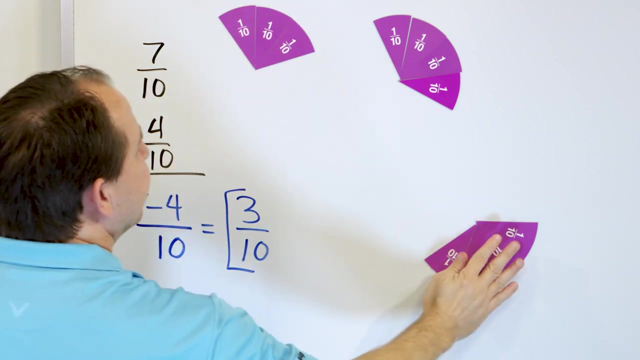 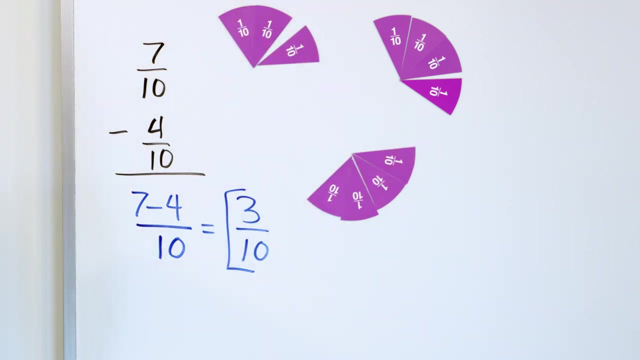 What this thing is saying here is if you start with this much pizza, 7 out of 10 slices, and you subtract 4 out of 10 slices, subtract this much, then it would be starting with this and taking away this amount of pizza and pulling it away. What do you have left? 3 out of 10 slices. If you start with this amount, and you take away the 4 slices, you have 3 out of 10. That's basically what that means. Now, I am going to go ahead and just kind of leave this up here. Well, kind of, why not? We can just leave it there. 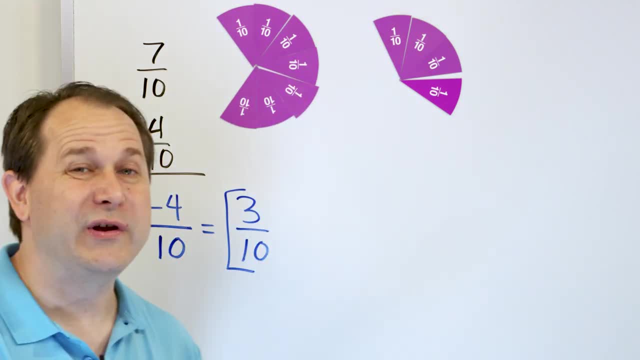 But we're not going to use the magnets anymore because it's very important for you to get good at this without, you know, drawing pictures. 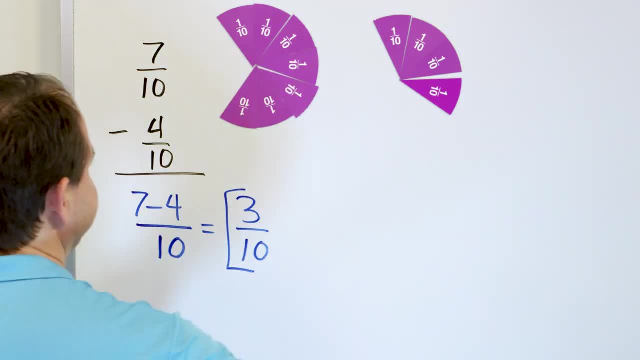 I think it's good to do, but we don't want to do it for every problem. 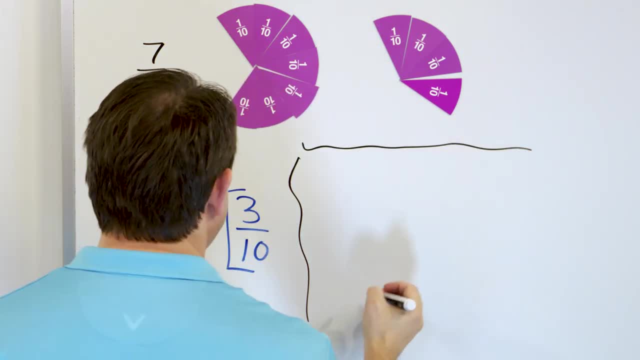 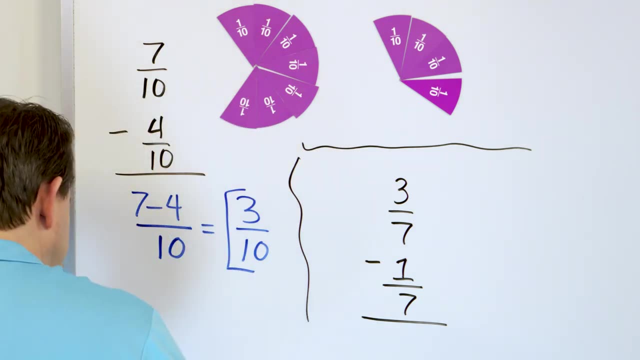 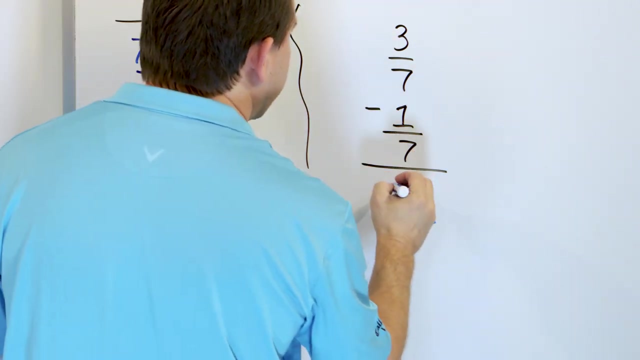 All right. Let's go over here and solve the next problem. Let's say we have 3 sevenths, and we'll subtract from it 1 seventh. All right. The denominator is a 7 and a 7, so the denominator is the same. We keep it in the answer. And we have a 3 and a 1, which means we subtract 3 minus 1. What do we have? 3 minus 1 is 2 out of 7. Can we simplify this? No, we can't. 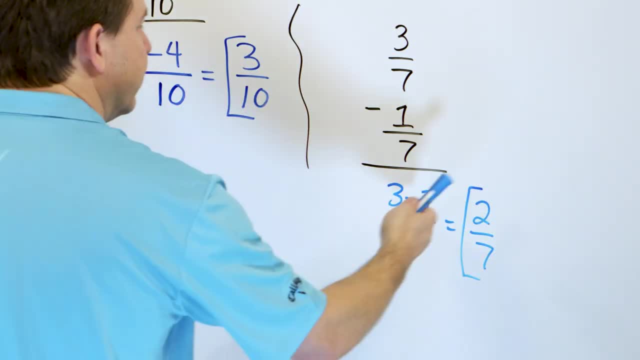 We can't divide top and bottom by anything else to make this simpler, so we keep the answer. It's 2 out of 7 pieces. Okay. That was problem number 5. Actually, that was the halfway mark. 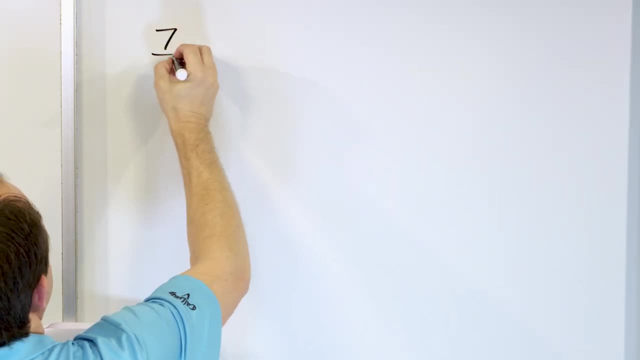 Let's take a look at problem number 6. Let's say we have 7 out of 12 slices of pizza, and we'll subtract 3 out of 12. 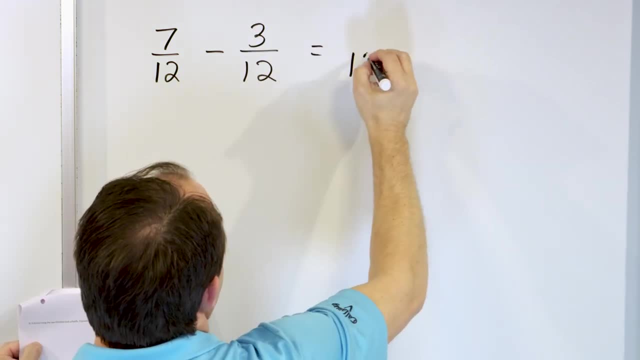 Now, the denominators are the same, so we keep it in our final answer. And then we subtract the top number, 7 minus 3. 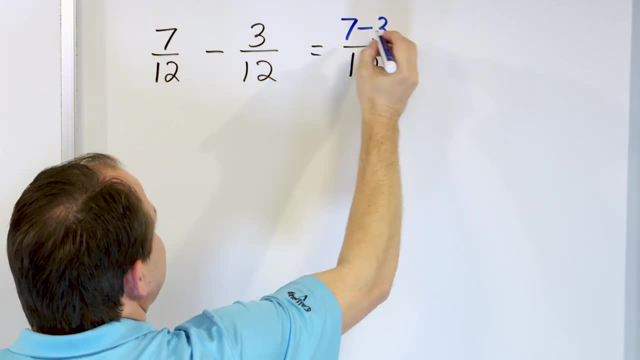 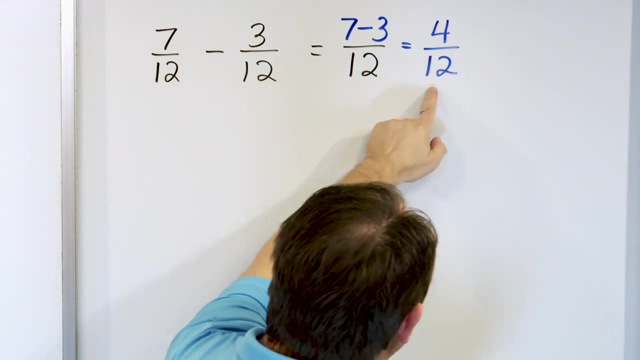 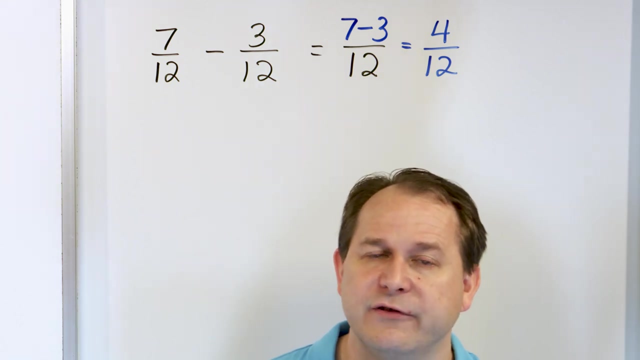 So over here, we'll have 7 minus 3. When you do 7 minus 3, what do you get? You get 4. And, of course, it's still out of 12 pieces. And then you ask yourself, can I simplify this? Can I divide top and bottom? Well, actually, I can divide top and bottom by 4. I could also divide top and bottom by 2. That's fine, too. 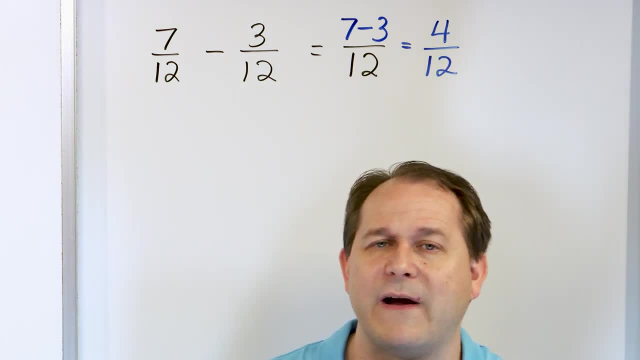 But if you divide by 2, then you'll get some other answer, and you'll be able to divide by 2 again. You'll have to do it 2 times. 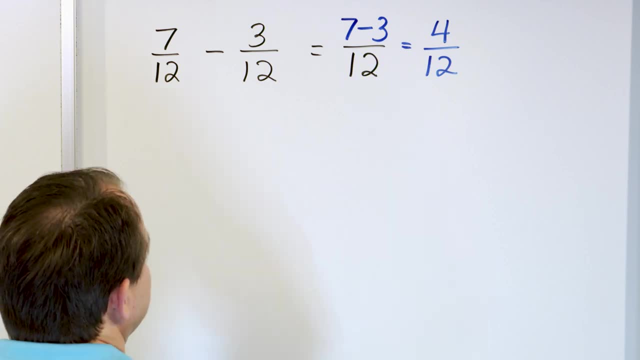 That's fine. There's nothing wrong with it. But let's, you know, let's just... 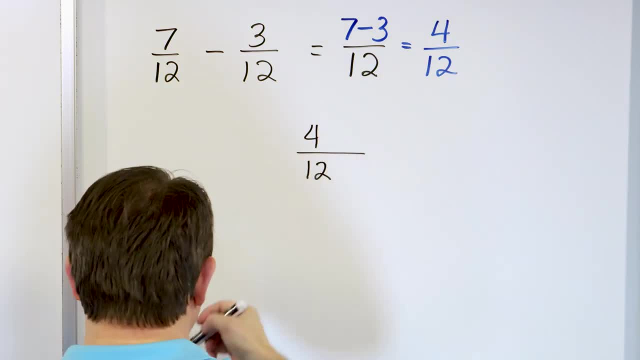 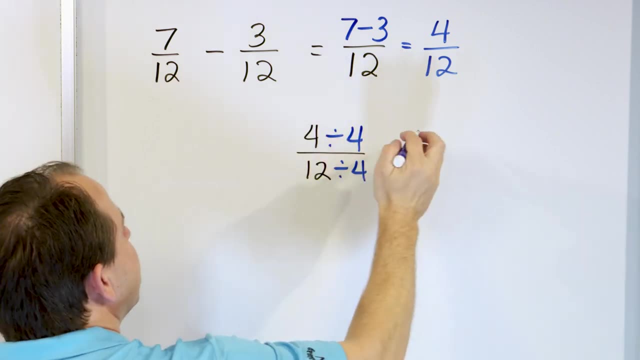 We can recognize we can take 4 twelfths and divide the top and bottom by a larger number. We can divide by 4. Both divisible by 4. 4 divided by 4 is 1. And 12 divided by 4 is 3. 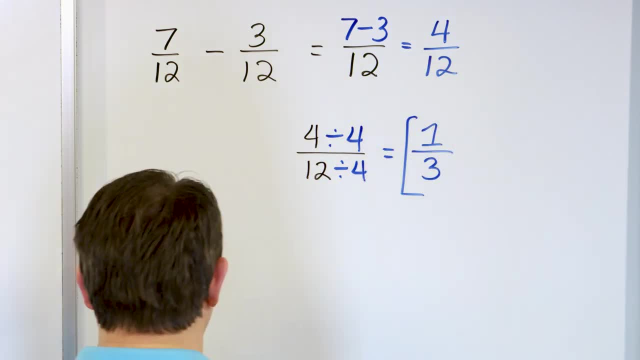 Because 3 times 4 is 12. And so the answer we get is 1 third. So if you start with 7 slices out of 12, and you take away 3 slices, then you're going to have 4 slices left. 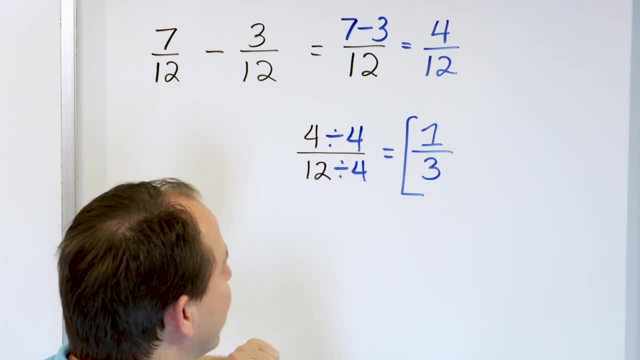 This is the right amount of pizza. But this is just a simpler way to write the exact same amount of pizza. So that's the final answer. 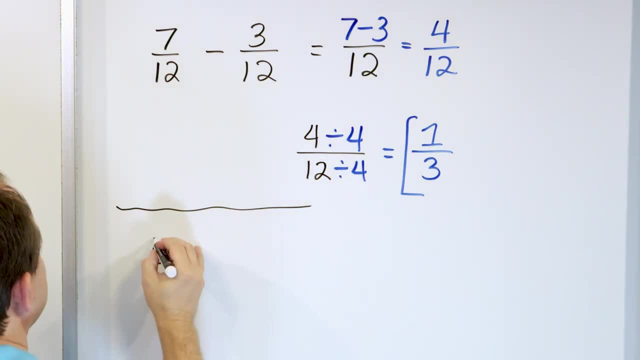 All right, let's take a look at problem 7. Take a look at 5 eighths. And we'll take away, subtract from that, 1 eighth. 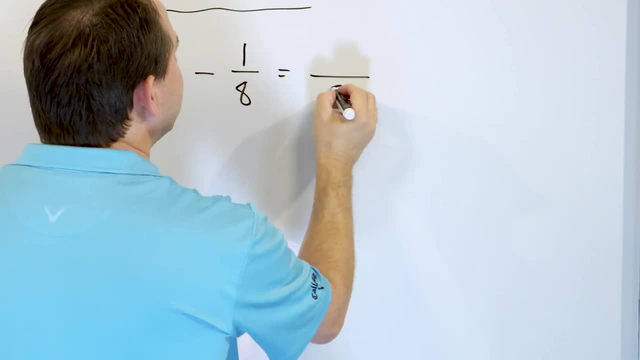 The denominators are the same. So because we're subtracting, we keep that in our final answer. 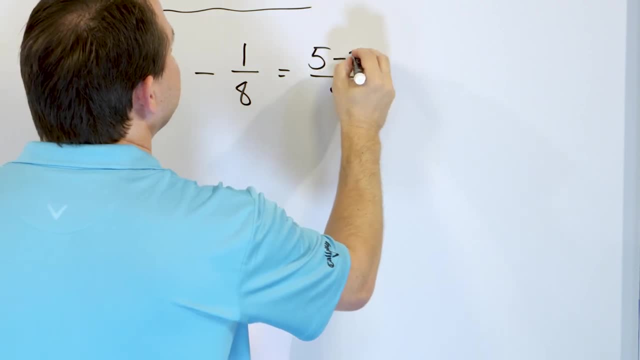 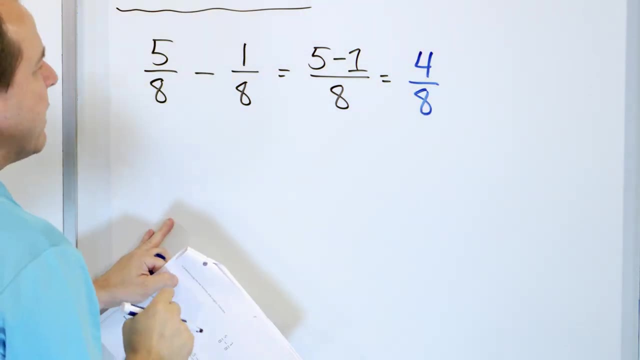 And we have 5 minus 1. So we have 5 minus 1 in the numerator. 5 minus 1, as you know, is 4. And then we have 8. Now can we simplify this? Well, we can divide top and bottom by 4. You could also divide by 2. 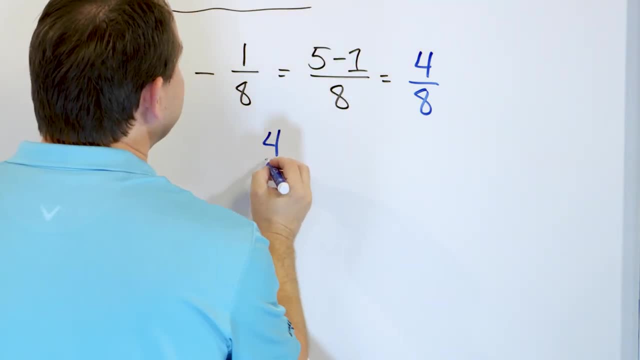 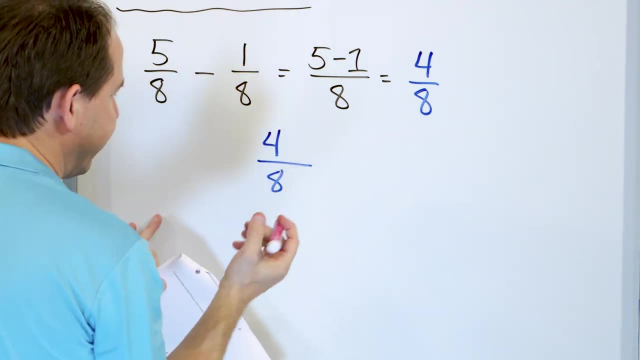 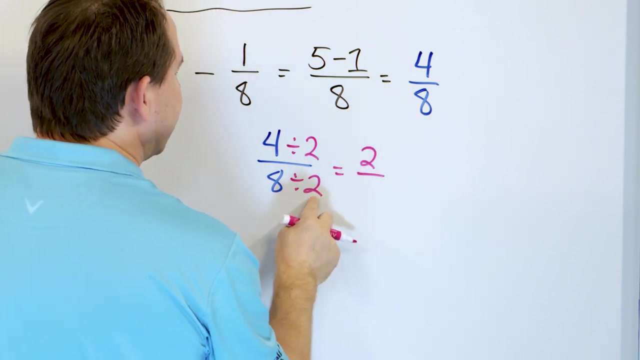 But then you would get something you would have to divide by 2 again. So let's do it that way. Let's not do the same exact thing every time. We know we can divide by 4. Because 4 certainly works. But let's divide by 2. Let's get some variety here. 4 divided by 2 is 2. And 8 divided by 2 is 4. 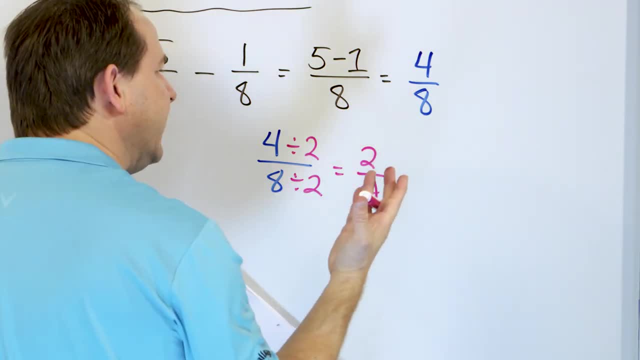 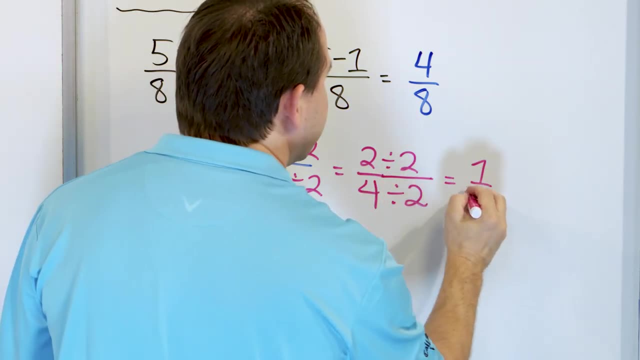 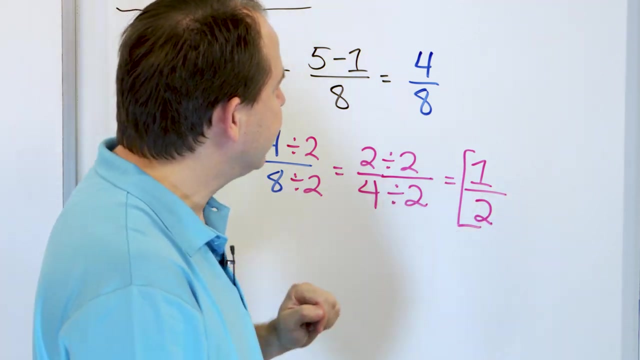 So we get 2 fourths. But we see, OK, we can divide by 2 again. So let's go ahead and divide this by 2 and divide this by 2. And 2 divided by 2 is 1. And 4 divided by 2 is 2. So you get 1 half. So is this fully simplified? Yes. I can't make it that any simpler. And you also should ask yourself, does it make sense? 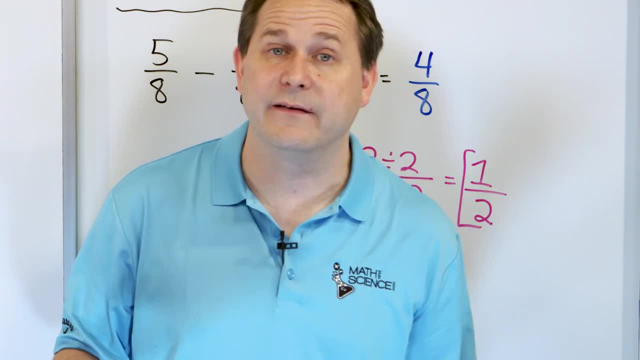 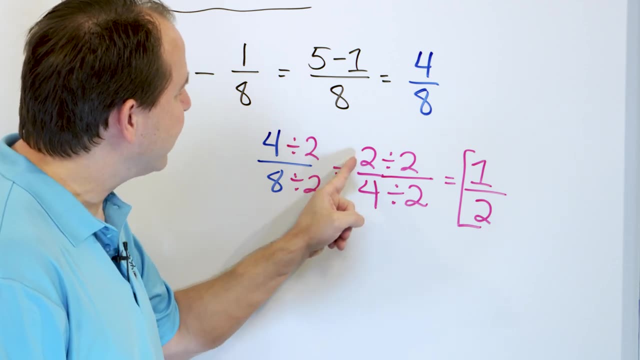 Well, what I got was 4 out of 8 pieces. If I have 8 pieces and I have 4 of those pieces, then I have half the pizza. That's what we have here. But that's the same thing as what we got here. 2 out of 4 pieces. We simplified it again. 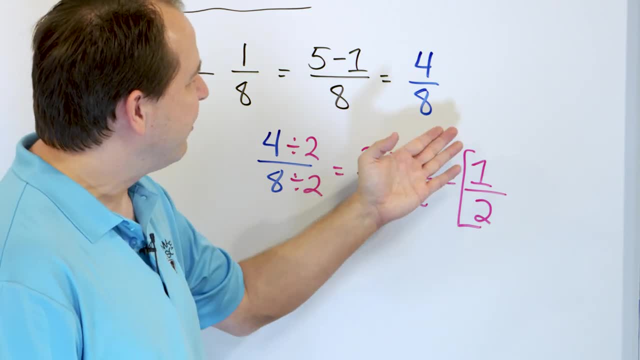 Here's 2 fourths is also 1 half, which is also 4 eighths is 1 half. It all means the same amount of stuff. It's just that the fraction looks a little bit different. All right. 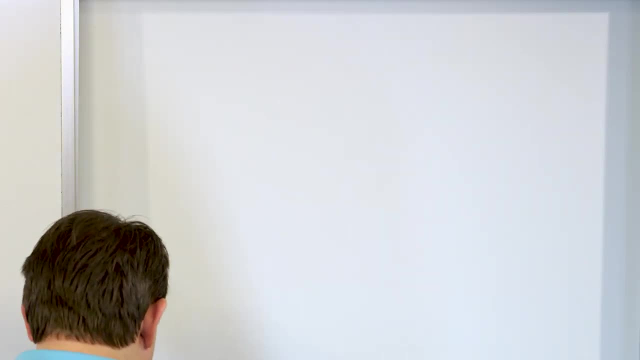 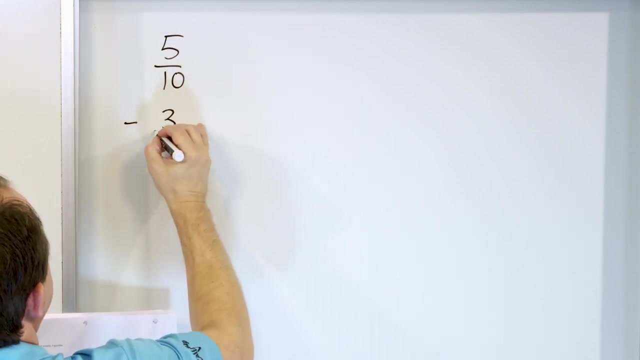 We have only 3 problems left. What do we have here? Let's take a look at 5 tenths. And we'll subtract from that 3 tenths. These denominators are the same. They're 10. So we keep the denominator the same at 10. 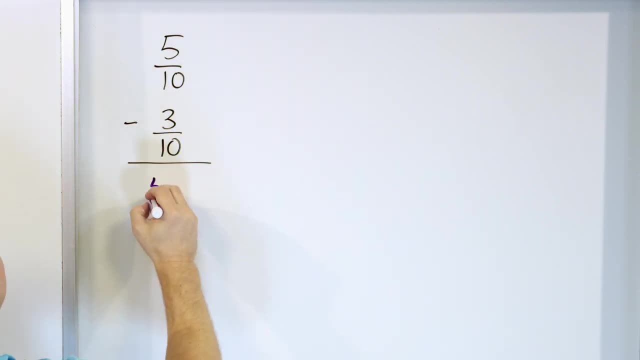 And we have a 5 minus 3 in the numerator. 5 minus 3. What is 5 minus 3? That's going to be 2. 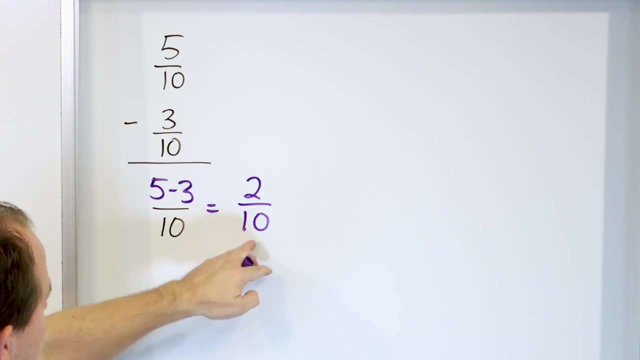 And then you have 10 here. Now, this is the final answer. That's great. But can you simplify it? Yes, you can. 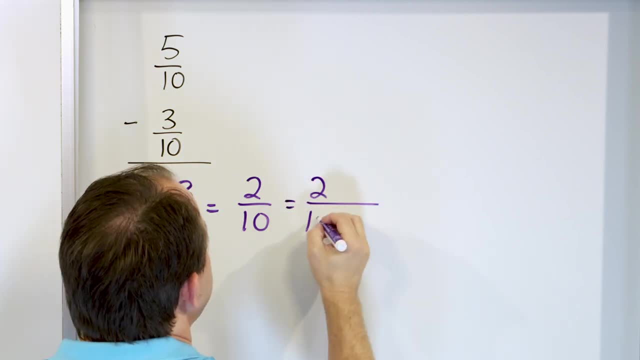 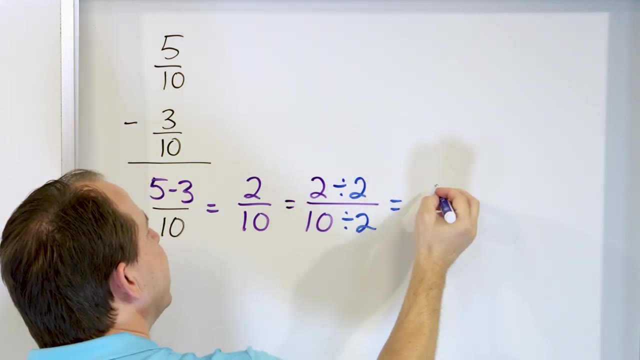 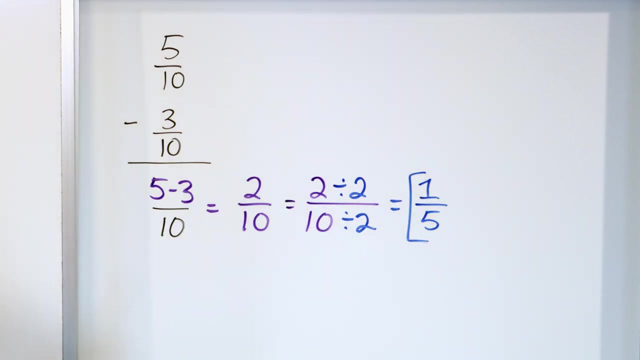 They're both divisible by 2. So we'll take the 2 tenths. And we'll divide the top and bottom by 2. We can divide this by 2. We can divide this by 2. 2 divided by 2 is 1. 10 divided by 2 is 5. And so the answer is 1 fifth. We get 1 fifth for the answer. 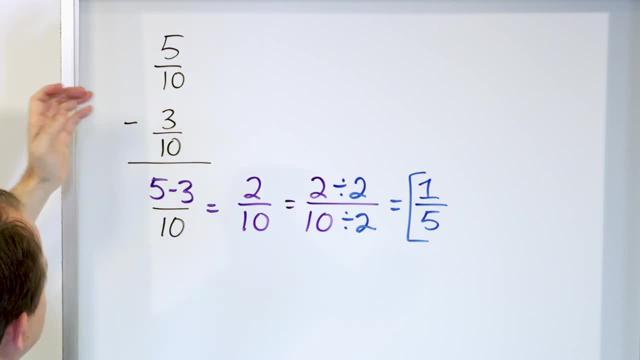 So if you start out with 5 pieces out of 10, and you take away 3 pieces or slices, then you will only have 2 slices left out of a 10-slice pizza. 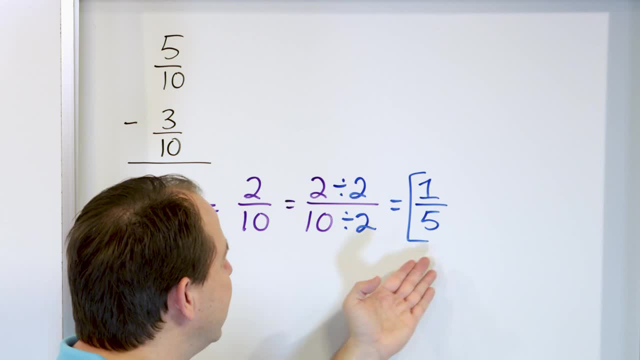 Right. That's correct. But a simpler way of writing the same amount of pizza is just to cut a new pizza into 5 slices and only take 1. It's the same thing. All right. So home stretch. Only 2 more problems. And here's the next one. 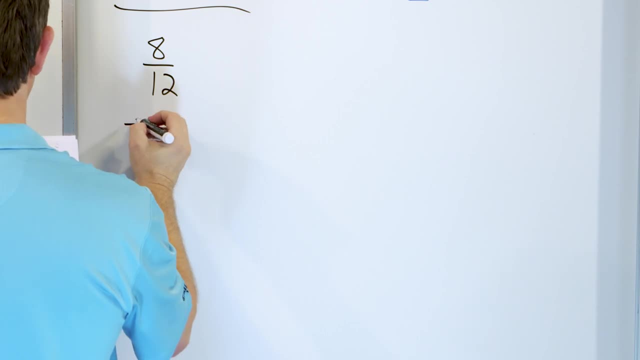 What about 8 twelfths? And we'll subtract from that 3 twelfths. The denominators are the same, which is 12. So we'll go ahead and keep that in our final answer. In the numerator, we have 8 and a 3. And it's a minus, so it's 8 minus 3 in the numerator. 8 going down 7, 6, 5. 8 minus 3 is 5. And you get 5 twelfths. Can you simplify this? 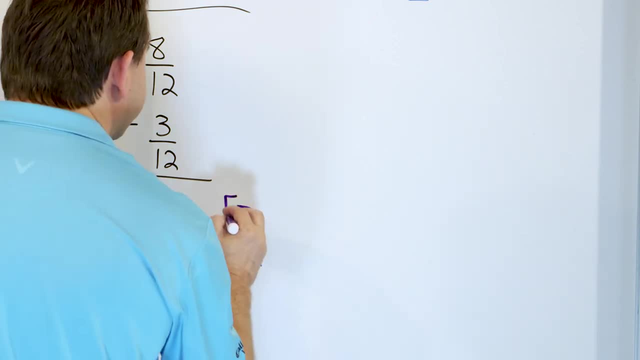 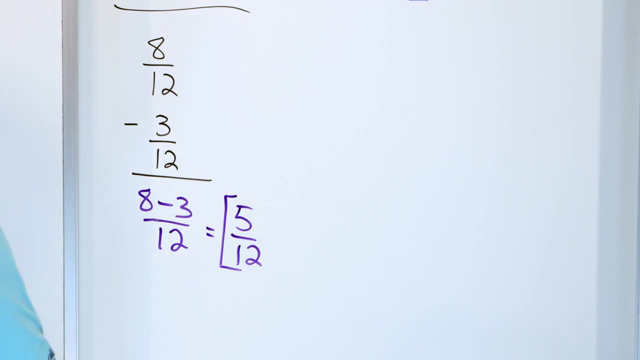 No, we can't. We cannot divide top and bottom by something to make these numbers simpler or smaller. And so we just say 5 twelfths is the final answer. All right. Now we have our very last problem. 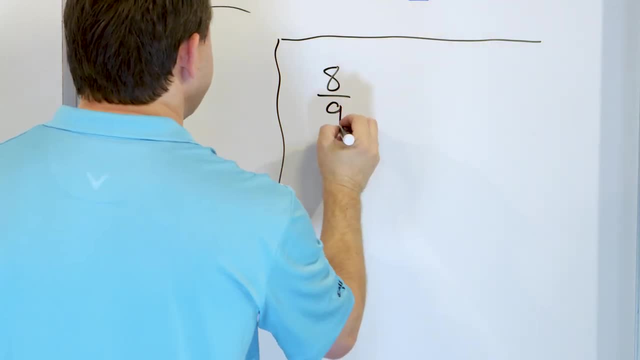 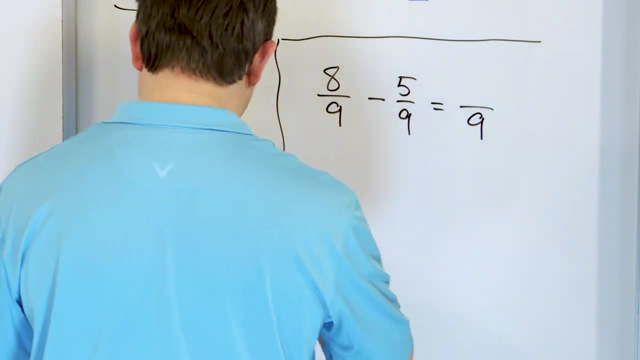 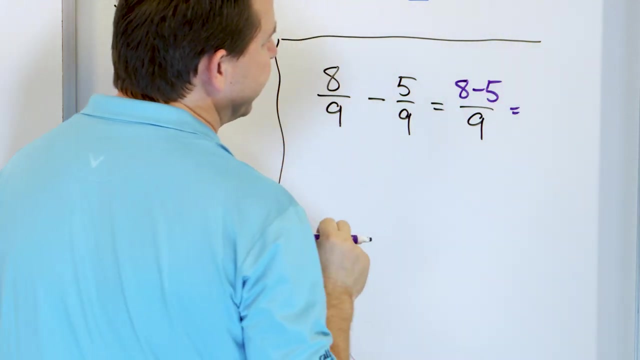 We have 8 ninths. And we're subtracting from it 5 ninths. First thing we check, are the denominators the same? Yes, they are. So we keep it in the final answer. And then on top, we have an 8 minus 5. So we write that as 8 minus 5. What is 8 minus 5? When you subtract that, you get a 3. 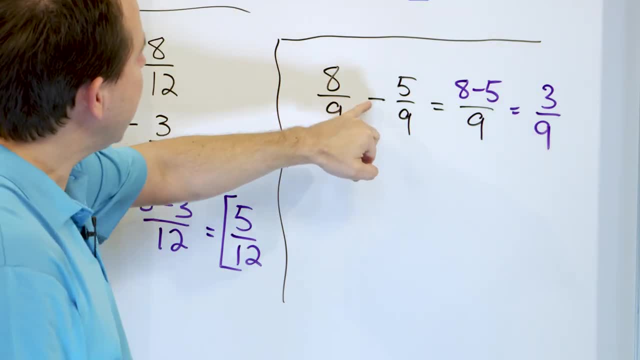 And you get, of course, out of 9 pieces. So if you start with 8 pieces out of 9, and you take away 5 pieces, of course, when the pizza is sliced into 9 pieces, you will have 3 pieces left. 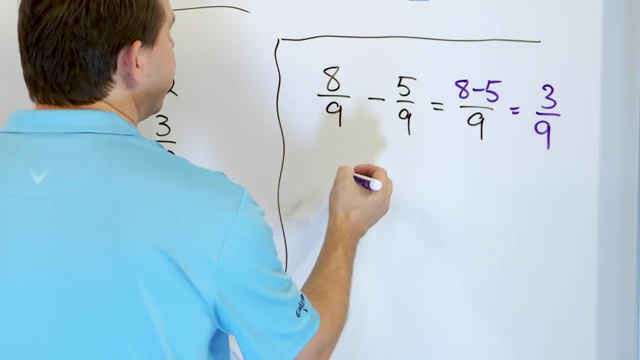 But this can be simplified. We can divide top and bottom by 3. So let's take that 3 ninths. And they're both divisible by 3. 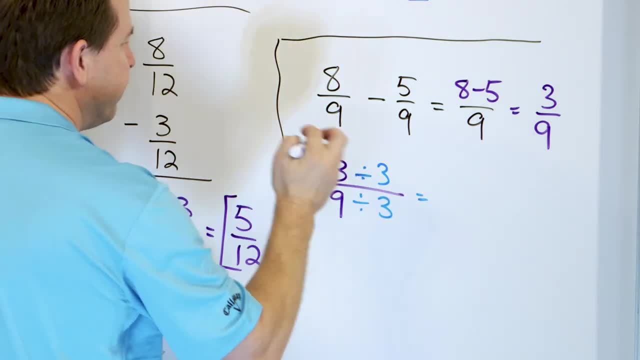 So we'll divide by 3, divide by 3. 3 divided by 3 is 1. And 9 divided by 3 is 3. So you get the answer of 1 third. 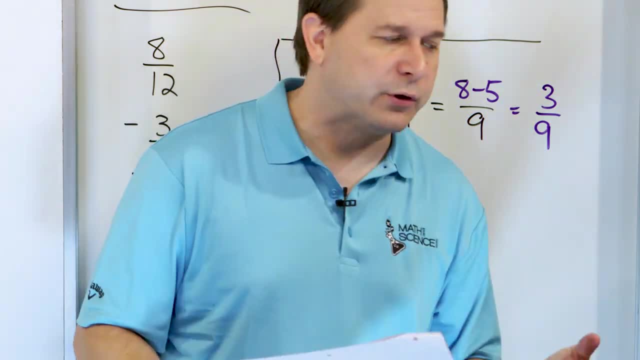 So the answer we got of 3 ninths is correct. But to make it simpler, this is a simpler way of writing the same exact amount of pizza. And you write that as 1 third. 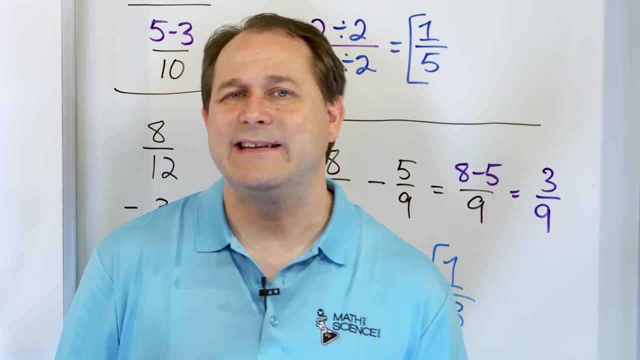 So here we have conquered the idea of subtracting fractions with like denominators. 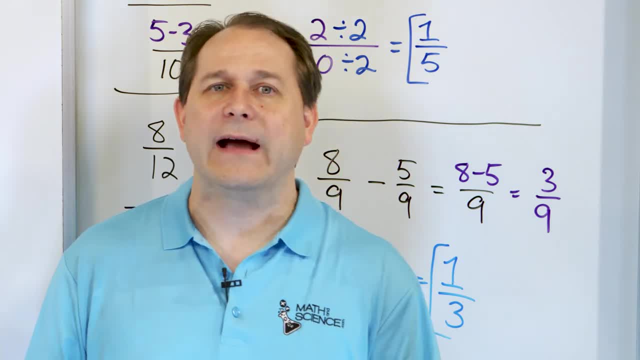 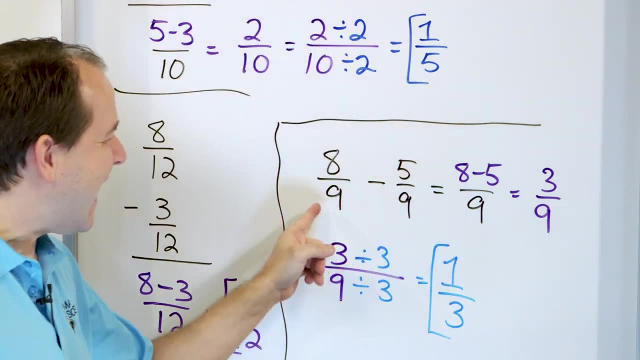 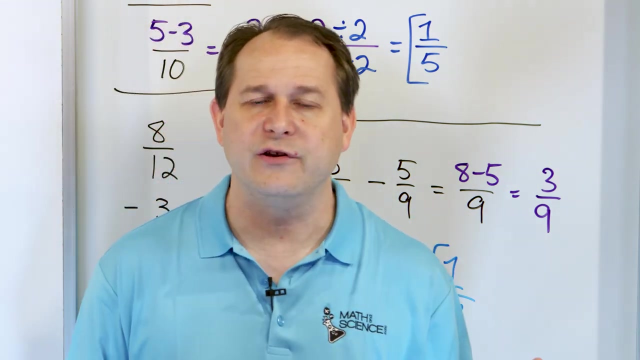 You can see it's the same process as addition. Other than the fact that when we subtract, we have to subtract the numbers on top, the numerators, instead of adding them. So denominators have to be the same to subtract them, just like for addition. And we keep the same denominator in the answer, just like addition. And we just subtract the numerators and simplify the answers. 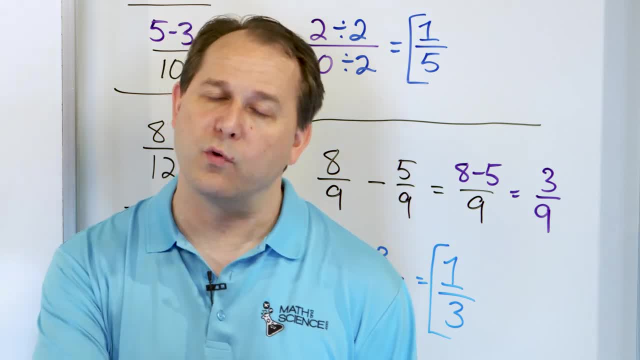 So I'd like you to practice all of these yourself. Follow me on to part 2, and we'll wrap up the concept of subtracting fractions when they have like denominators. 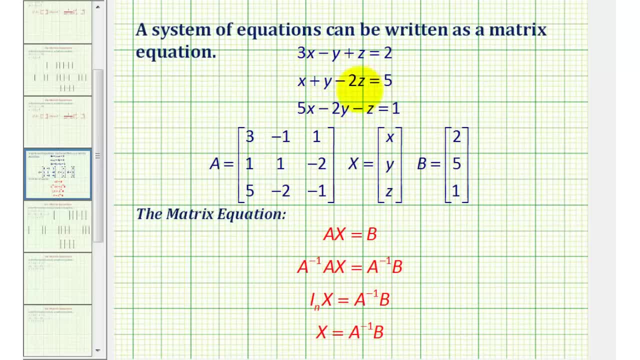 form, meaning we have the x terms, the y terms and the z terms on the left side of the equation and the constants on the right. Once the equations are in the correct form, we're going to form three matrices. Matrix A will be the coefficient matrix. matrix X will be the variable matrix.